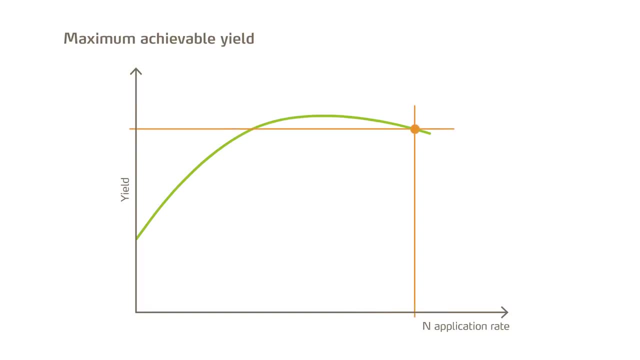 One of the key findings of a nitrogen response curve is its summit. It corresponds to the maximum achievable yield. The corresponding nitrogen supply rate is also called the agronomic optimum. In reality, a farmer needs to maximize returns, not yield. This situation is described here. 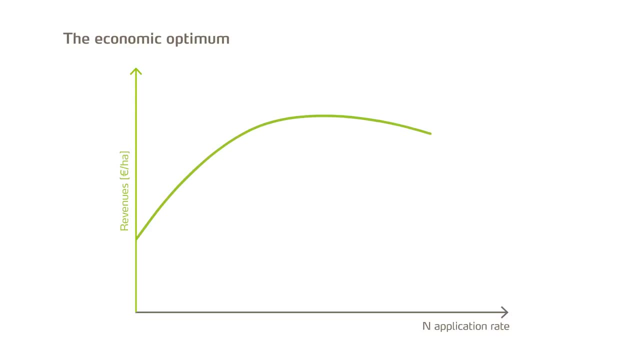 The yield is now indicated in euros per hectare. Likewise, the cost of fertilizer is indicated in euros per hectare. The more fertilizer is applied, the higher the cost. With increasing N application rates, farmers generate additional returns, as long as the additional revenue grows faster. 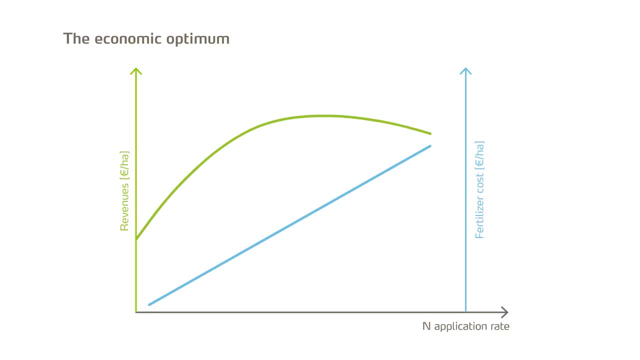 With increasing N application rates, farmers generate additional returns as long as the additional revenue grows faster than faster than the cost of applied nitrogen. In other words, maximum returns are obtained when the slopes of the green and blue curves are the same. This is called the economic optimum. 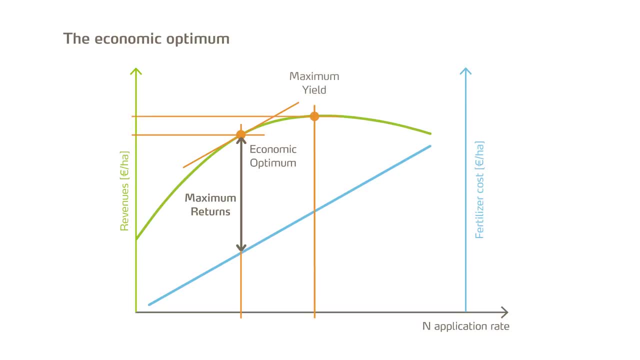 The economic optimum is always lower than the maximum yield. Environmental regulations might reduce application rates even further, preventing the economic optimum from being reached. Mobile applications愀 only possible by many uses. Market prices of crops and fertilizers have an impact on the economic optimum. 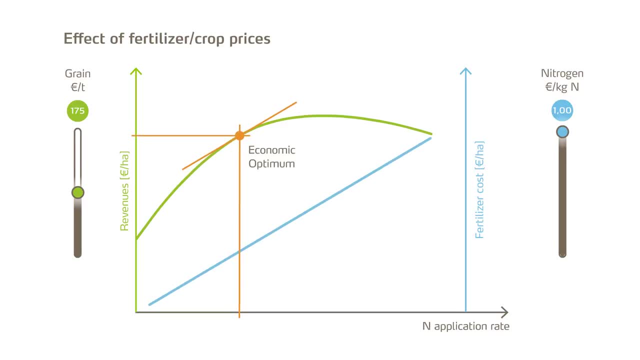 When fertilizer becomes more expensive, the slope of the blue line becomes steeper and the economic optimum shifts to the left. Vice versa: when the cost of fertilizer decreases, the economic optimum shifts to the right. When grain prices change, revenues are impacted and the green curve moves up or down accordingly. 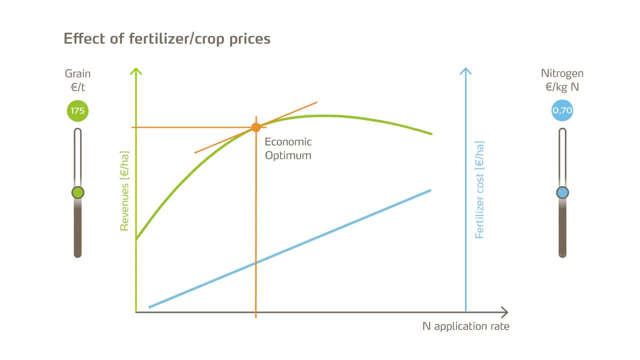 Other factors, such as crop quality, may have an impact on revenues. For example, if a certain protein level needs to be achieved, increasing nitrogen supply might be beneficial When comparing the impact of different parameters such as nitrogen form on yield and returns. 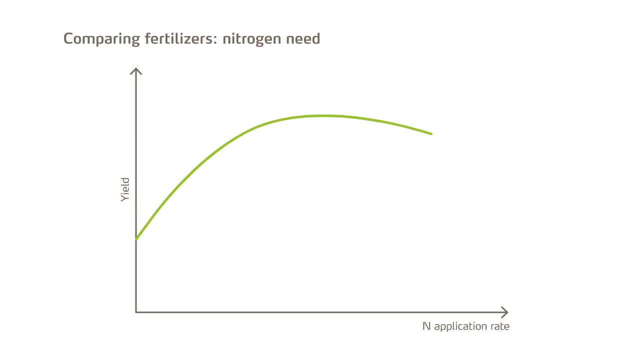 we have to compare them. We have to compare the corresponding response curves. Let's assume the dark green curve corresponds to ammonium nitrate and the light green curve corresponds to urea. The same yield can be achieved with both fertilizers in this example. 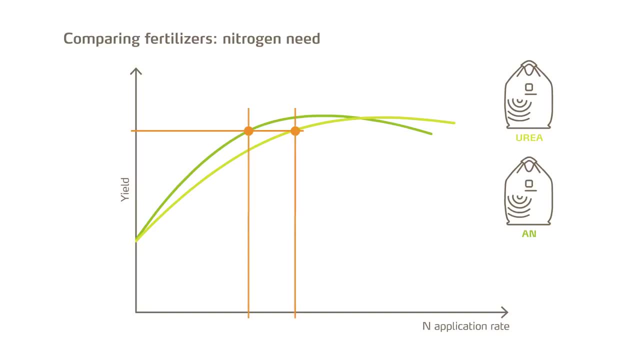 However, significantly more nitrogen is needed with urea than with ammonium nitrate. The difference is due to the higher nitrogen uptake efficiency of ammonium nitrate and the lower losses. Likewise, for a given amount of nitrogen, yield and revenues will be higher with ammonium nitrate than with urea. 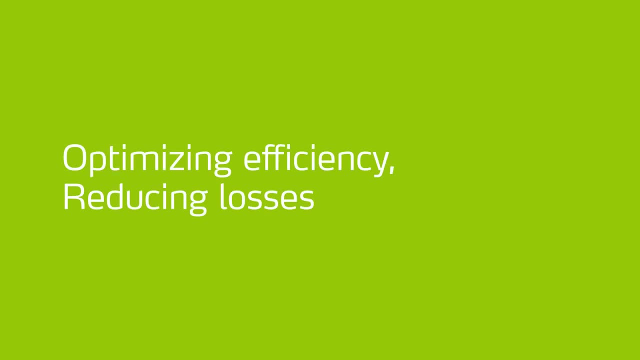 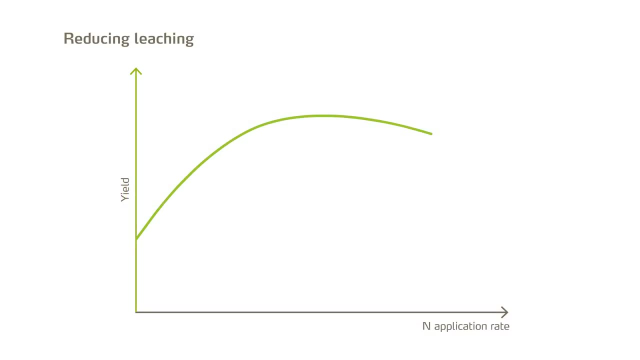 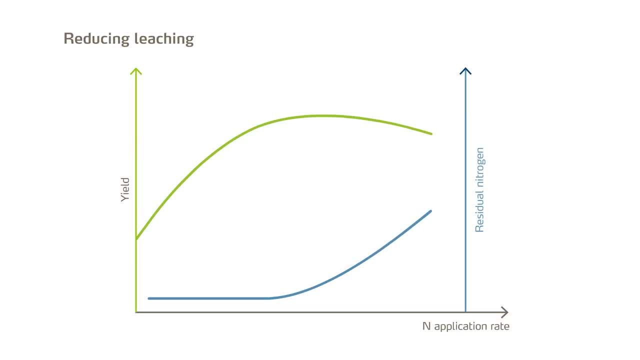 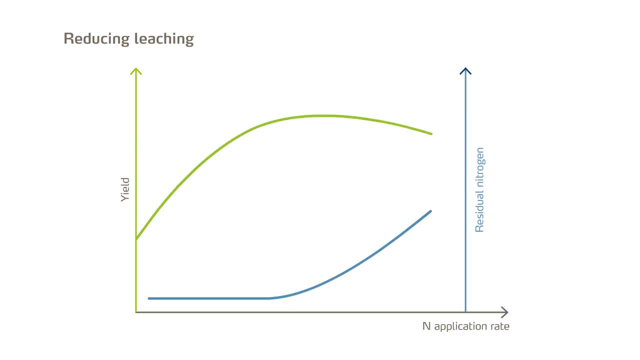 During the growing season, crops take up water and nitrogen from the soil at high rates. Leaching is most likely to occur during heavy rainfall in autumn and winter. For nitrogen application rates below the maximum yield, the risk of leaching in winter is low. 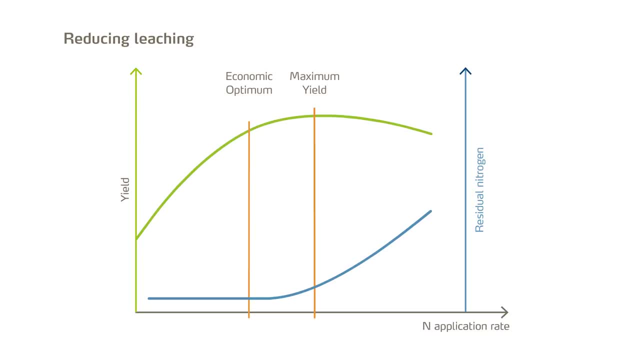 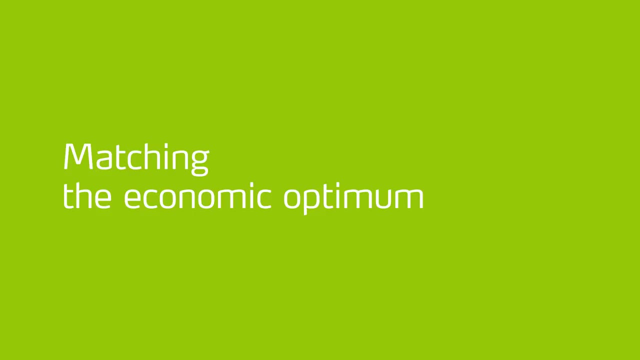 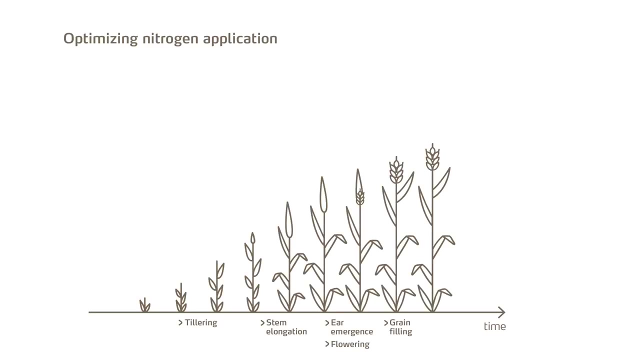 since the crop will will have absorbed almost all of the available nitrogen in the soil. Response curves help to validate and calibrate precision farming tools so that the economic optimum can be reached under all circumstances. Crop nitrogen demand depends on the yield objective and is determined by weather conditions and crop health. 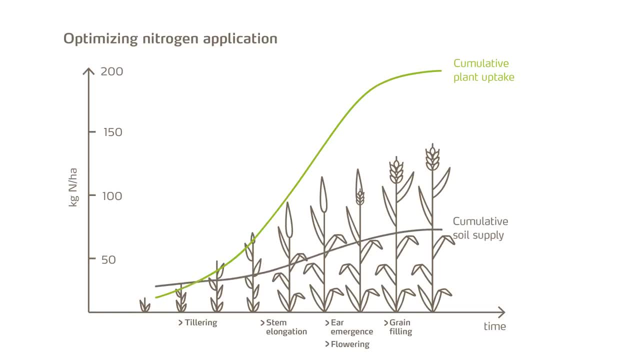 Soil nitrogen supply depends on weather conditions, organic fertilizer application and soil conditions. Fertilization needs to fill the gap between soil nitrogen supply and plant needs. In practice, fertilization is tailored to actual plant needs during the entire growth season by split application. 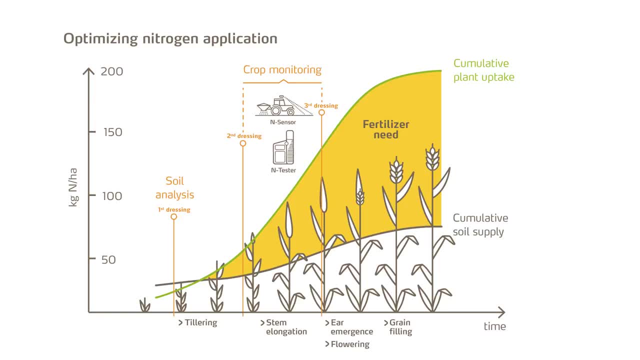 Precision farming tools such as the N-Tester and the N-Test and the N-Sensor measure the actual nitrogen status of the crop. They enable precise prediction of the amount of nitrogen required to match the economic optimum. Precision farming techniques are most efficient with fertilizers.